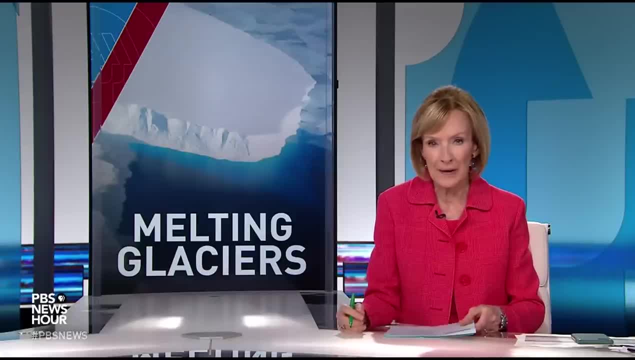 JUDY WOODRUFF, The New Yorker" In addition to its connection with the extreme heat and weather events here and around the globe, climate change is also having a measurable impact on a much slower-moving development: the loss of glaciers and the melting of the 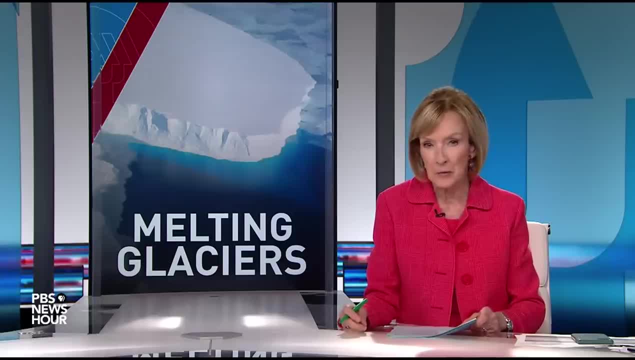 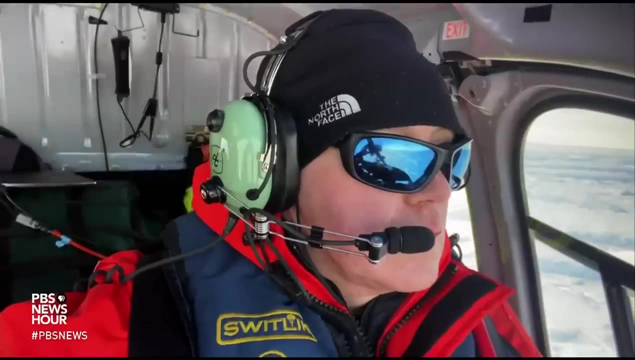 ice Science correspondent Miles O'Brien has been chronicling one scientist's quest to track what's happening with one of the most important glaciers. Here's his latest update: MILES O'. It was like a scene from Star Wars when climate scientist David 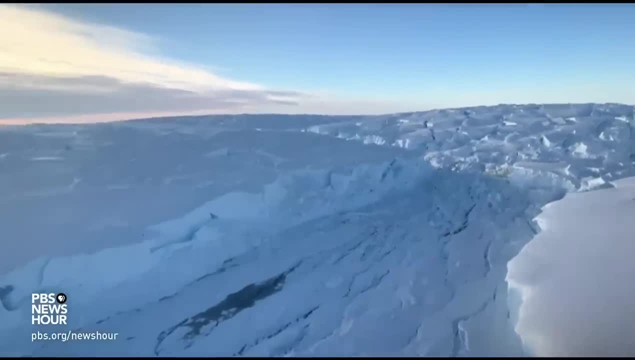 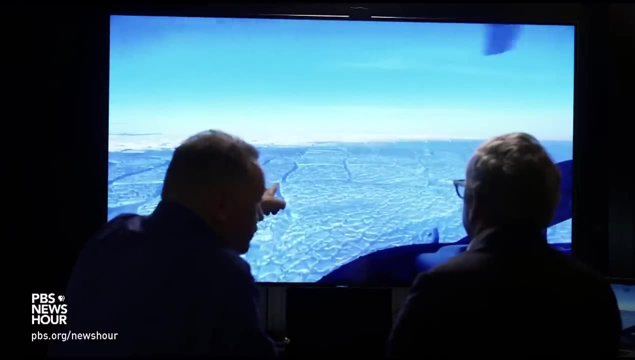 Holland finally made it to ground zero. DAVID HOLLAND- Just absolute insane fun And I actually thought I was going to die. We flew the helicopter through those crevasses. MILES O' These ice canyons are in the Thwaites Glacier in Antarctica. It's the 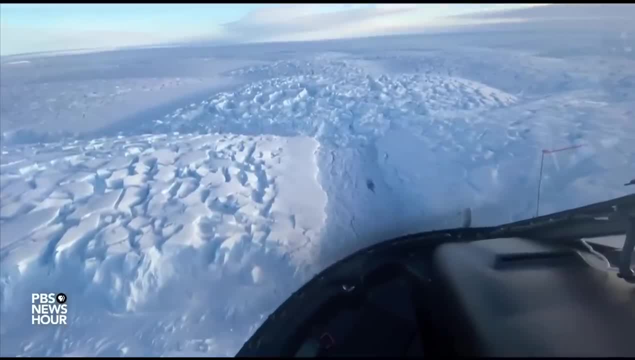 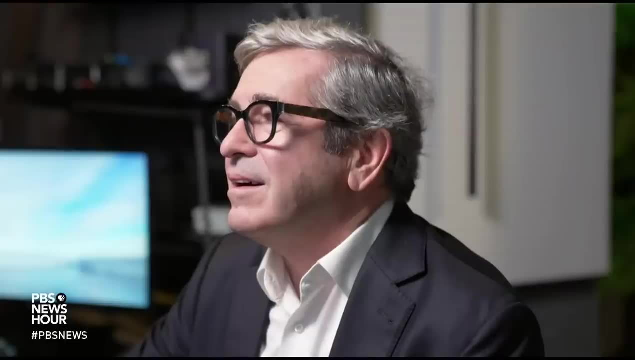 so-called Doomsday Glacier And you are seeing it in its death throes as close as anyone ever had ever seen. DAVID HOLLAND. This is perhaps the most important glacier in the world in terms of its potential impact this century. 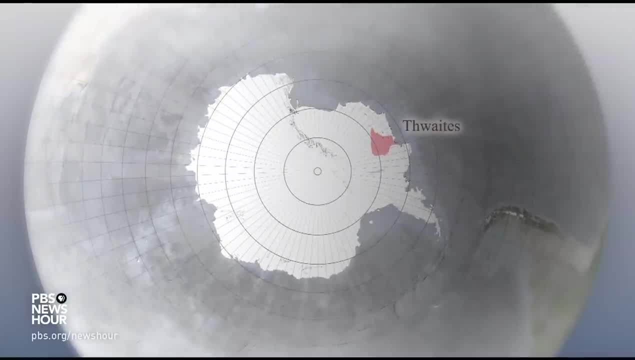 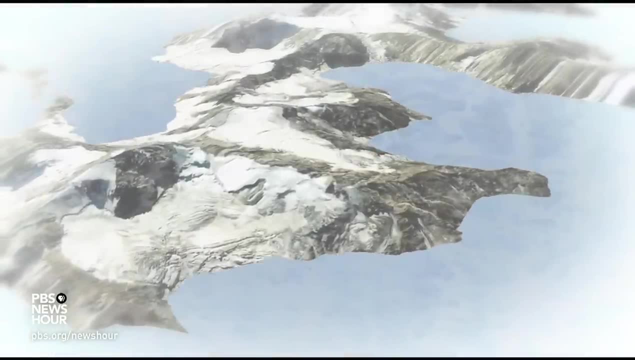 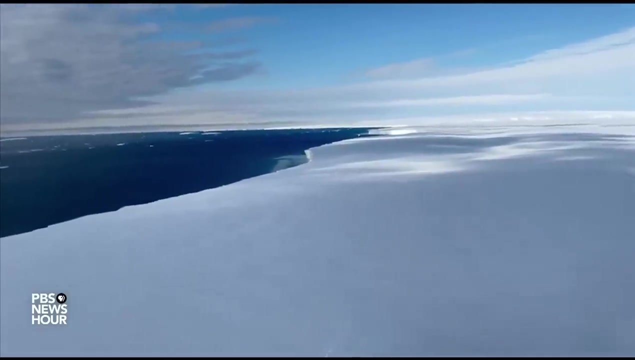 MILES O' The size of Florida Thwaites stores enough water to increase global sea level by almost three feet. if it all melted, 10 feet if the ice it helps hold in place slides into the sea behind it. And here the ice is melting at a stunning rate: 100 meters. 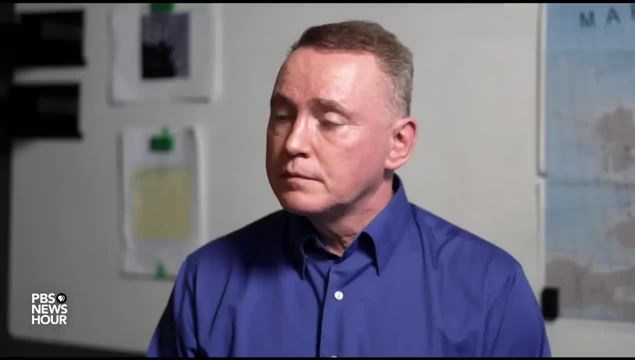 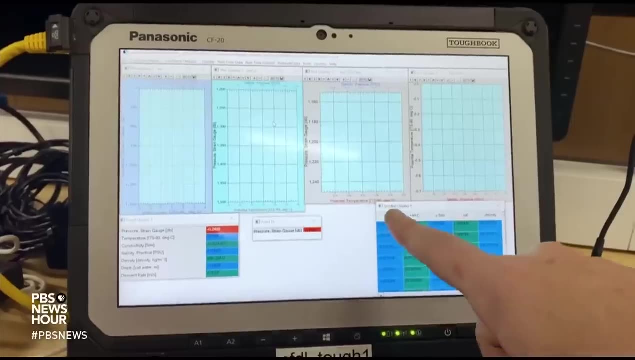 more than 300 feet a year. How long can it last? DAVID HOLLAND, That's an excellent question, And that's really the one we're pushing for. is we want to have, if you will, an ice forecast? 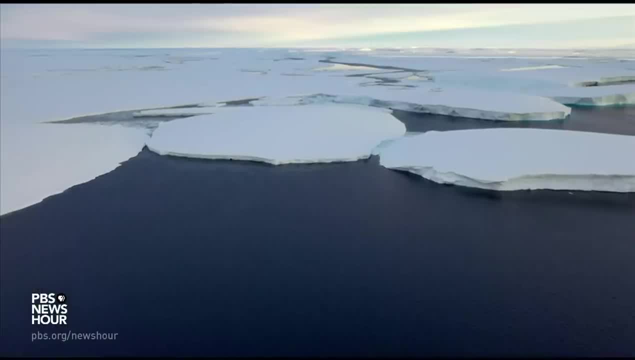 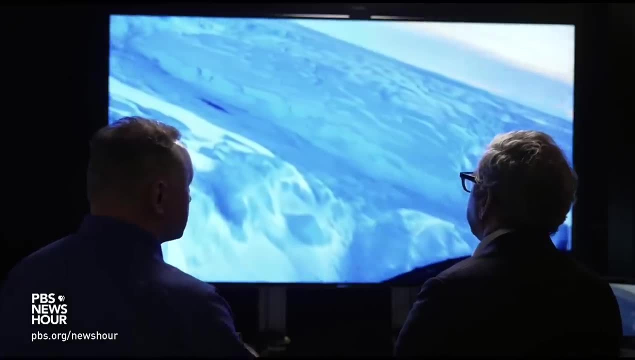 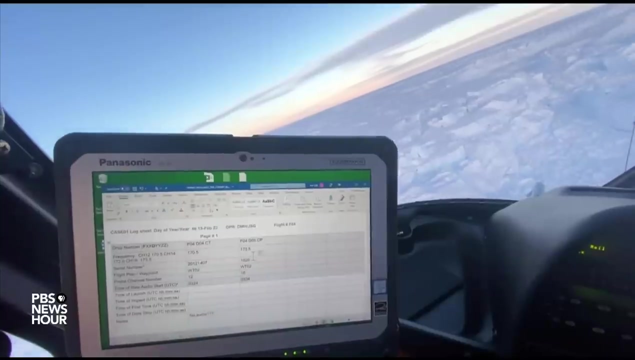 Without an ice forecast, which we currently don't have, we have really no insight into our future. MILES O' Holland is a professor at New York University. There we watch some scenes from his epic voyage. Year after year, he risks his life here and in the Arctic in pursuit of elusive data. 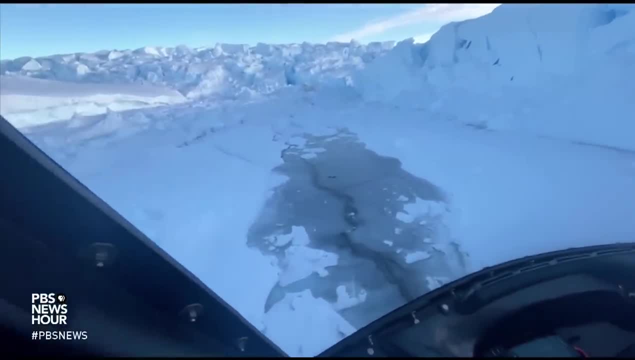 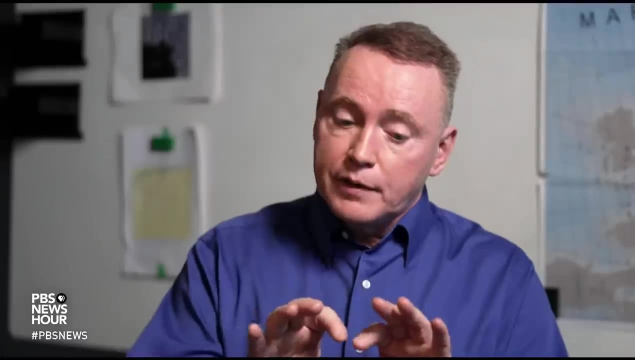 For starters, he wants to know the water temperature below these cracks. But the probe holding the instruments isn't breaking through. DAVID HOLLAND, There's a thin film of ice, maybe an inch or so. When you drop the probe, it hits the ice and it won't go through it. 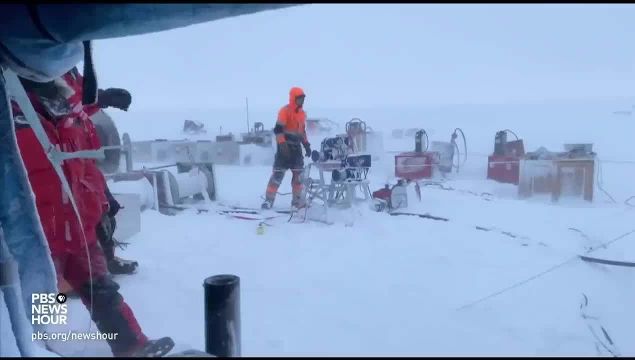 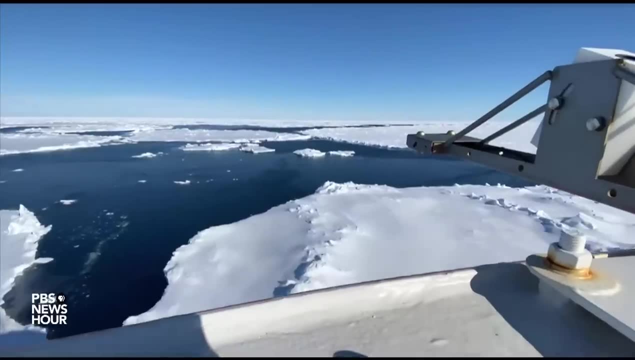 MILES O', Finding a way through that thin layer of ice was the umpteenth challenge in a litany that he encountered during this long, unpredictable and yet serendipitous Antarctic campaign. DAVID HOLLAND, This was the most difficult mission we have ever been on. 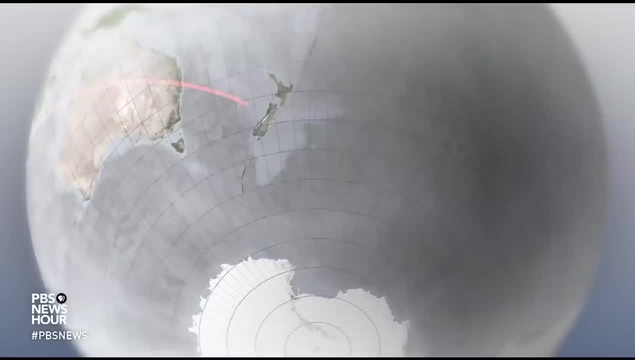 MILES O'. This was the most difficult mission we have ever been on MILES O' They arrived in Christchurch, New Zealand, on December 20.. It took three weeks for their COVID quarantines to lift and their equipment to arrive. 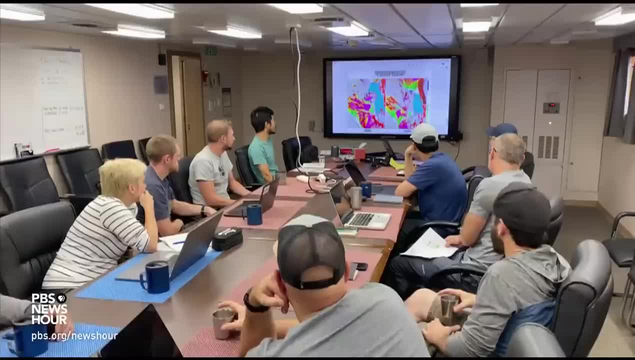 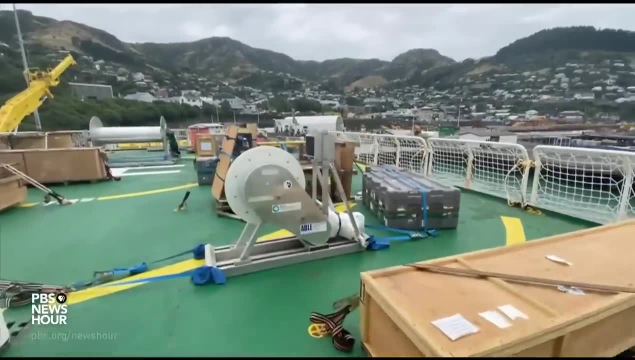 Ready to set sail next week? Yes, MILES O', All right, MILES O'. Funded by the National Science Foundation and its counterparts in the UK, Canada and South Korea, three dozen researchers boarded the South Korean icebreaker Ariane. 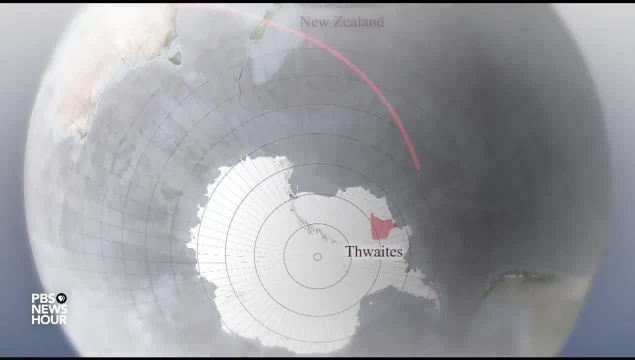 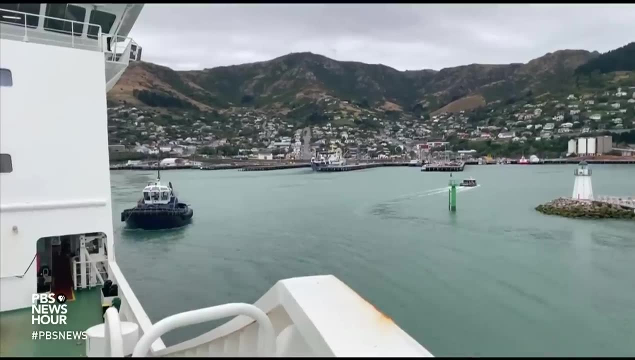 Brimming with gear. the ship set course for Thwaites, 3,000 miles away, DAVID HOLLAND. This idea was just go straight to the ice shelf. And it turns out that brilliant idea led to failure because we weren't planning on sea ice. 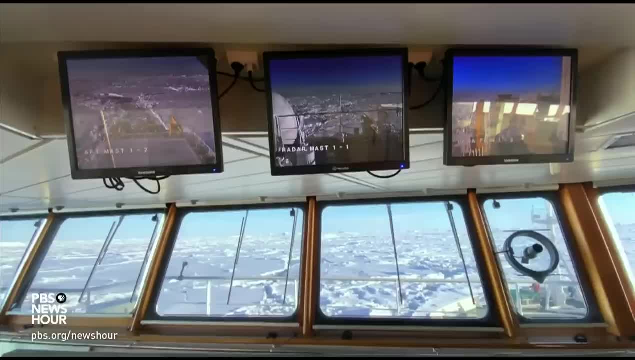 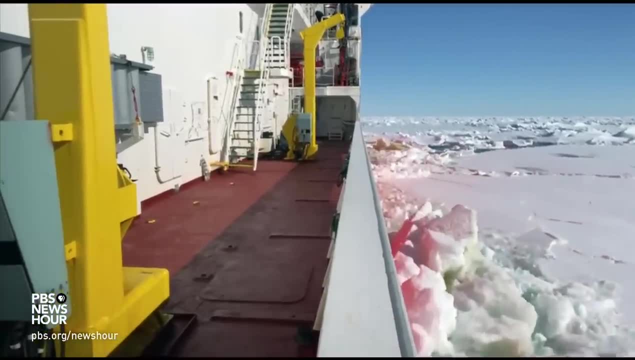 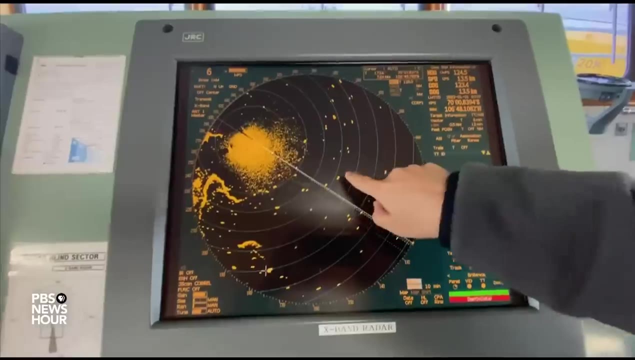 MILES O' Ariane is a Korean portmanteau meaning all seas. Seemingly true to her name, the ship cuts through most ice like butter at 14 knots. most ice. For unknown reasons, a huge conglomeration of sea ice floated in the Amundsen Sea between them and 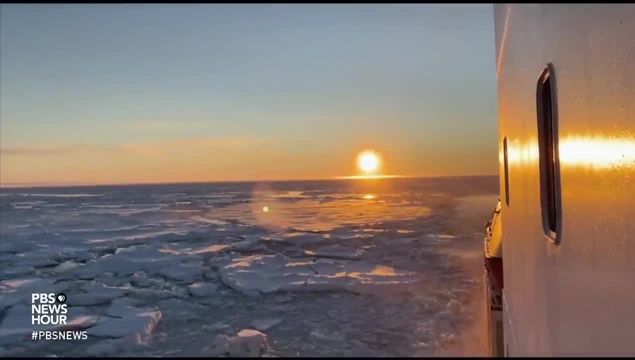 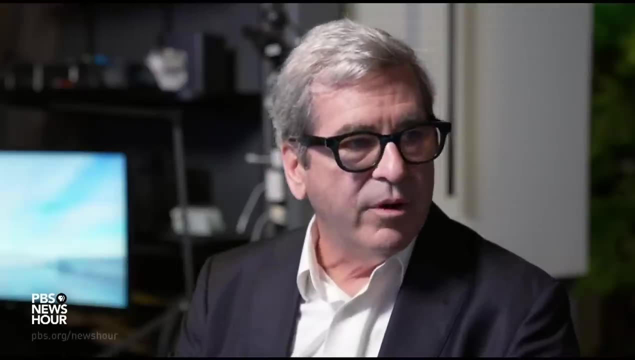 Thwaites. Eventually, it was too much for the Ariane. DAVID HOLLAND, The dreams of reaching Thwaites have pretty much been dashed now, MILES O'. What are your thoughts at that point, DAVID HOLLAND, That we have lost the prize actually? 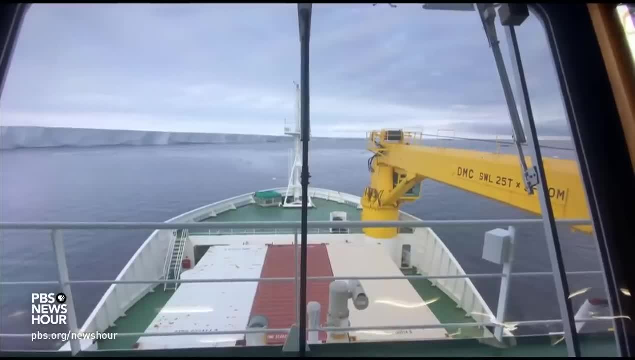 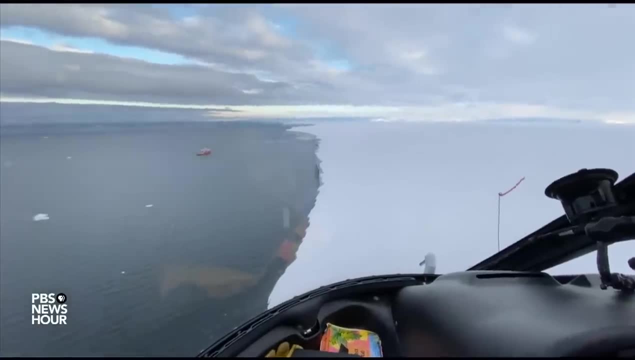 We were not going to be able to do this and we were not going to get that data. MILES O' All geared up with no place to go. Team Holland started eyeing a consolation prize. DAVID HOLLAND, It's Monday morning, January 24.. We arrived here. This is the Datsun Ice. 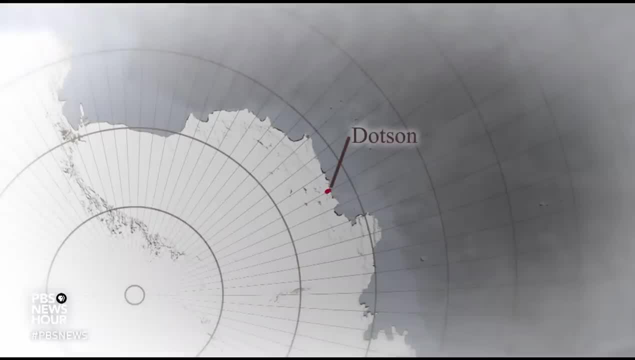 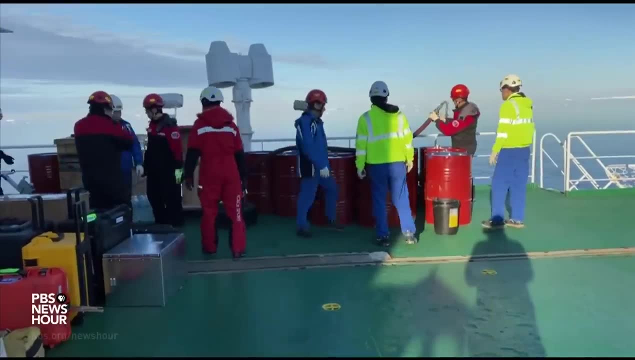 Shelf MILES O' The Datsun Ice Shelf is stable, not a heavyweight global threat like Thwaites, but it is a local target of opportunity. So they got busy deploying the scientific field camp they had designed for Thwaites on Datsun. 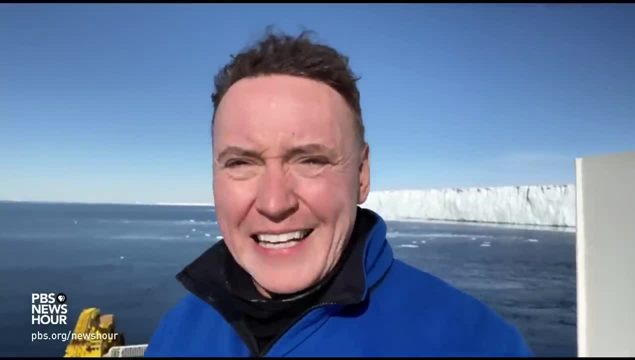 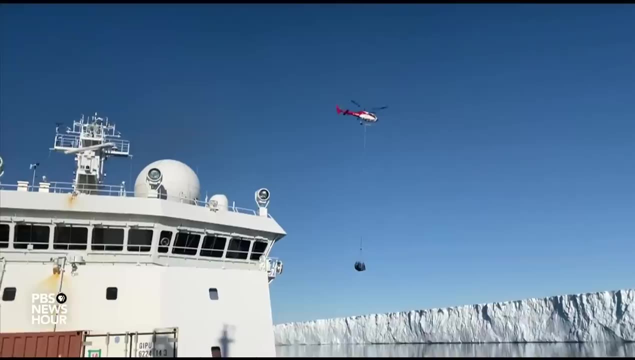 DAVID HOLLAND. All the helo operations are moving at lightning speed. MILES O'. They had to airlift 50 tons of gear, one ton at a time. DAVID HOLLAND, Equipment and people are shuttling off the ship to our base camp. 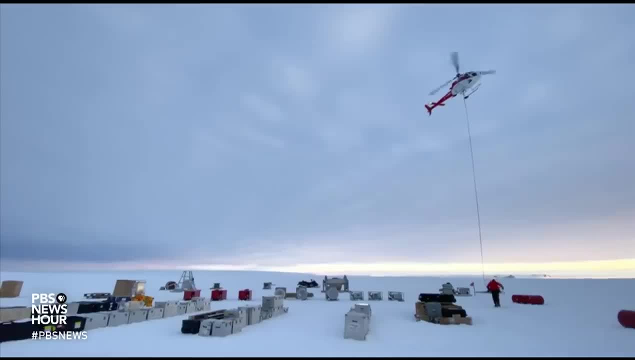 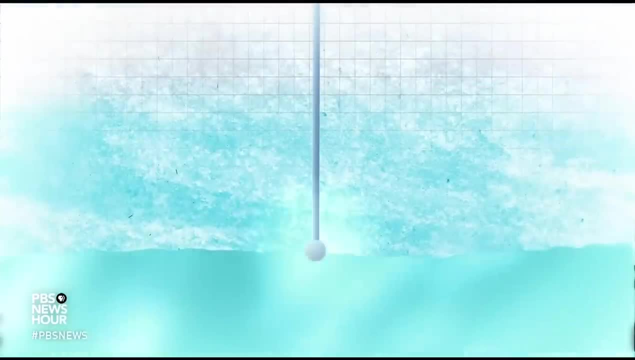 about 20 kilometers inland behind me, MILES O' The mission there, Drill a one-foot-wide, quarter-mile-deep hole through the ice to the sea beneath, drop instruments in and leave a mooring behind to monitor what is happening, where most of the melting occurs. 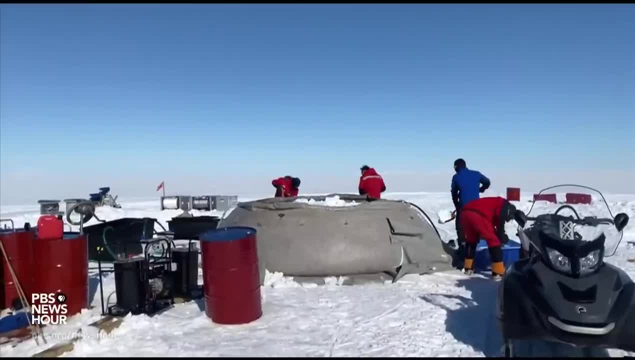 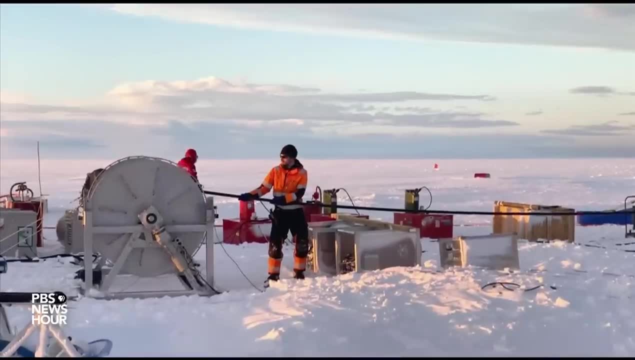 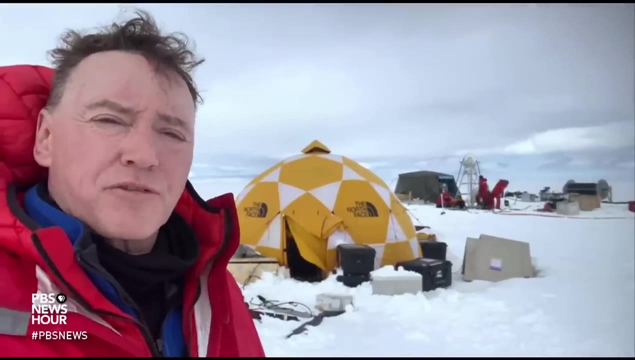 They drilled with hot water made from snow hand-shoveled into a 2,600-gallon container. As they set up the gear and started drilling, Holland scrambled to make his complex mooring work. The pressure was on DAVID HOLLAND, So the guys think they will be through in about six hours. 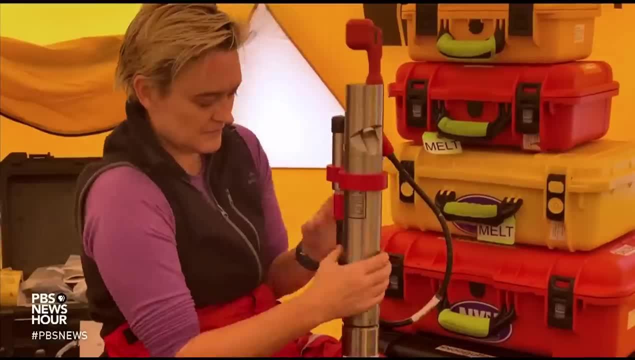 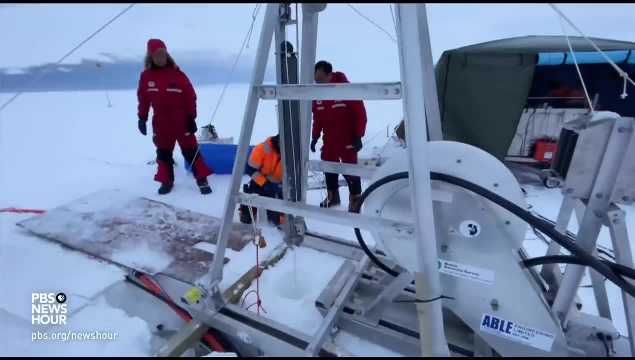 And after that we're kind of ready for the mooring. but the mooring is not really ready for them, MILES O'. Up until this point the weather had been benign by Antarctic standards- clear and cold. But on the day that everything had to be ready, 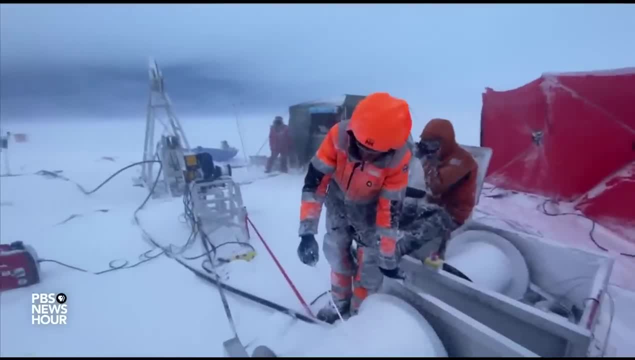 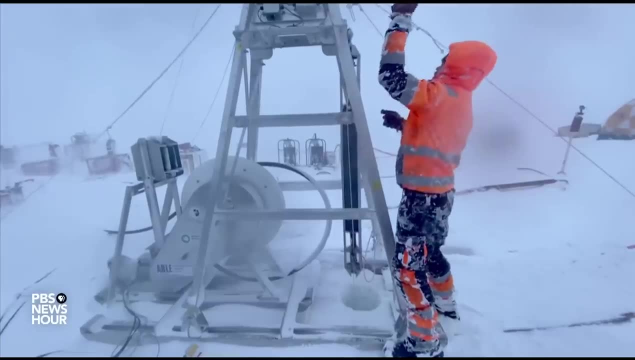 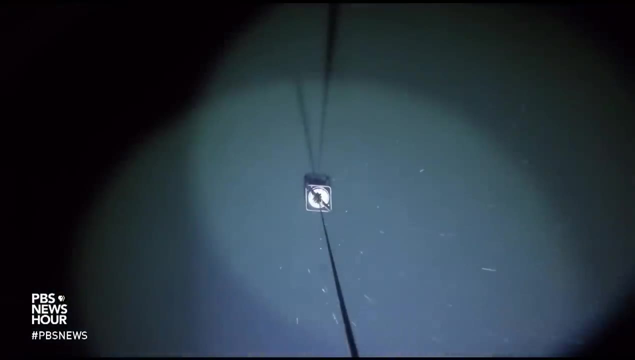 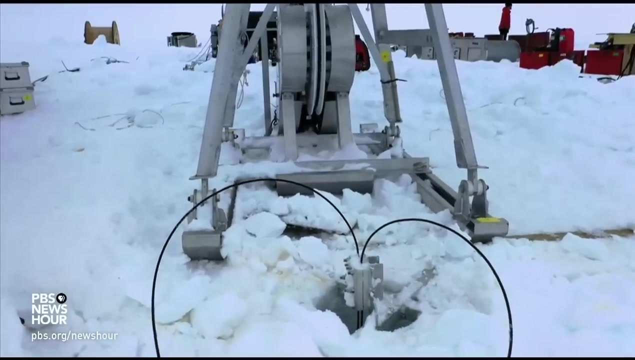 Early Monday morning, the weather has gone And now the snow is really starting to blow. There was no time to hunker down, So down went the mooring. fingers crossed, DAVID HOLLAND. It is Wednesday, February 10th. The mooring was installed and frozen in. 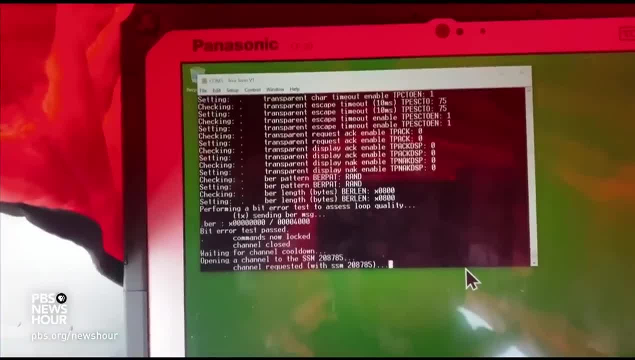 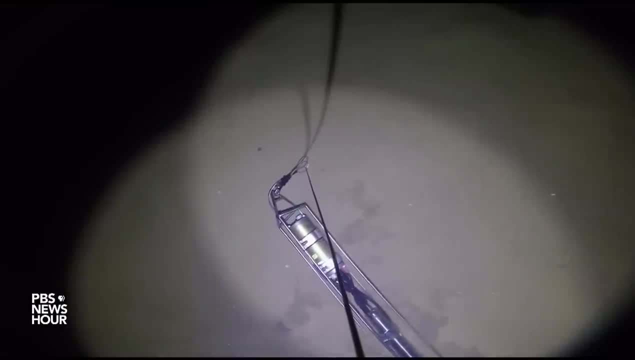 about a day and a half ago. Some 1,300 meters or 4,000 feet below me is an instrument that's talking right now with this computer: WOO-HOO, DAVID HOLLAND. Okay, Little bit of a restraint now. 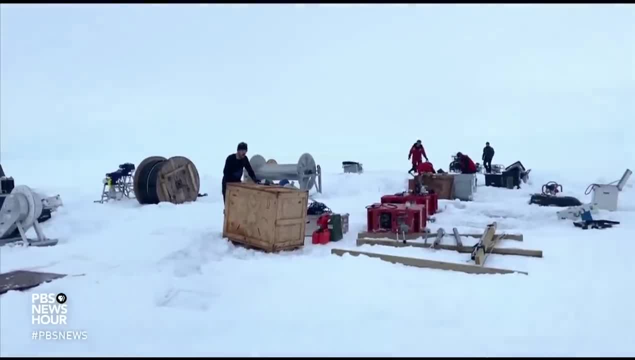 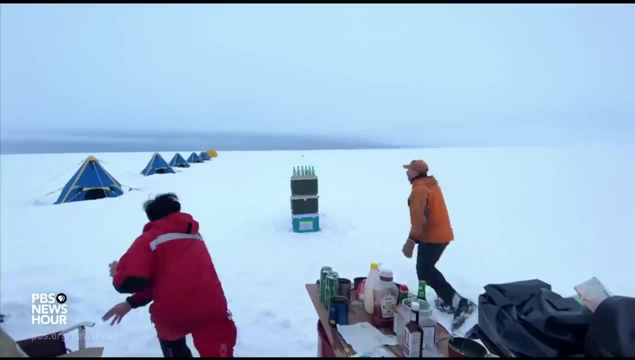 WOO-HOO, DAVID HOLLAND. Yes, WOO-HOO, WOO-HOO, DAVID HOLLAND. There was a lot of screaming and hoo-HA, Even though it was the middle of a blizzard. it was like this works. 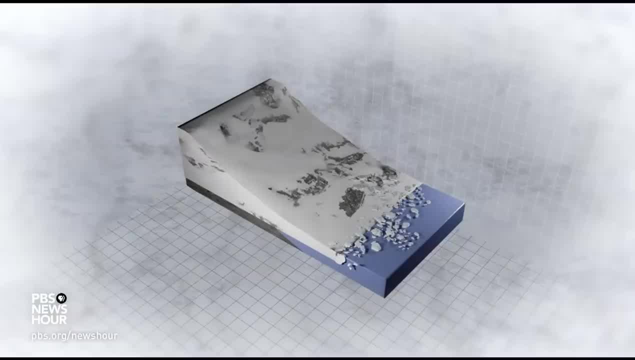 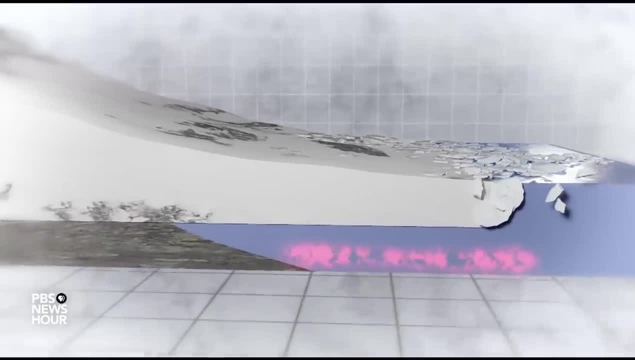 It was still the sense that we didn't achieve what we wanted. MILES O'. He wanted those instruments beneath Thwaites, at the place where the glacier meets the land. There, warm seawater interacts with cooler melted freshwater from the glacier, an area called the. 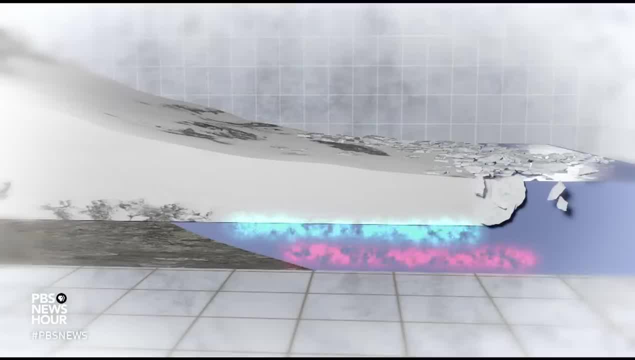 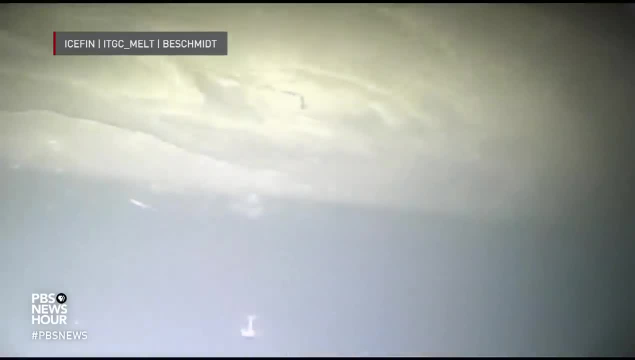 boundary layer. It creates turbulence, DAVID HOLLAND. So it's that turbulence at the boundary layer. that is how warm water from the ocean gets to the ice. It has to go through this boundary layer, but we don't understand the turbulence in it, so we want to capture it and see it.